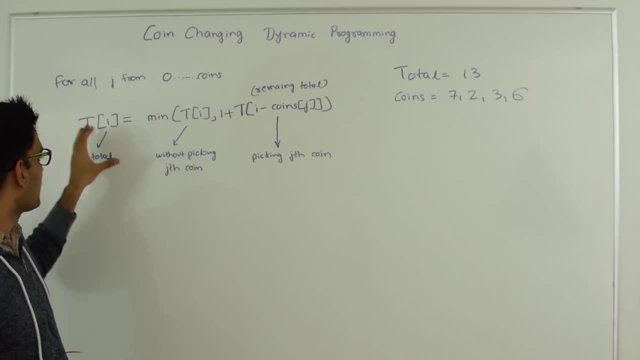 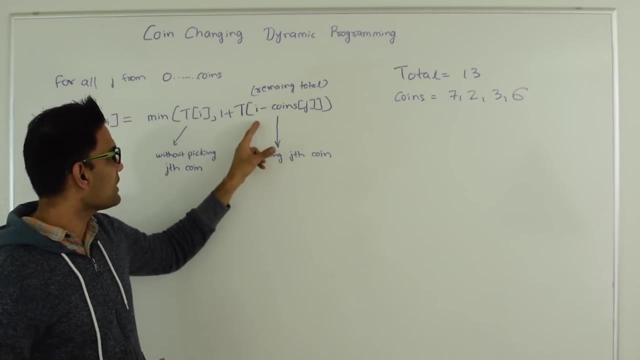 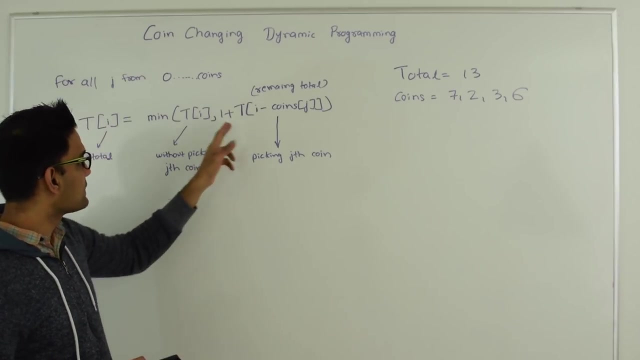 the jth coin. If you do not pick the jth coin, the value is same as old T, which is why this T. or if you pick the jth coin, you are left with i minus coins of j or i minus denomination of j total, and the minimum to form that total is T. So that value plus 1, because 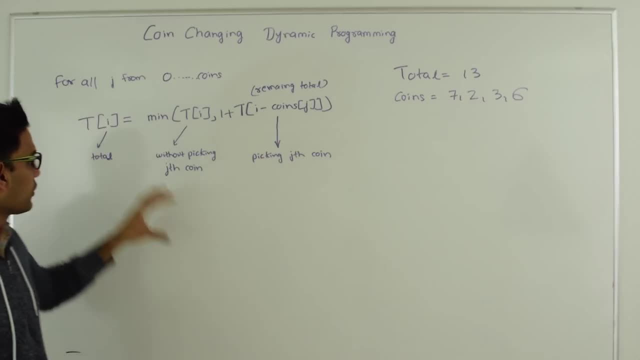 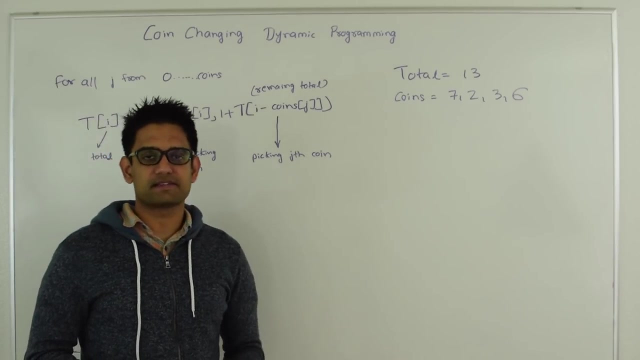 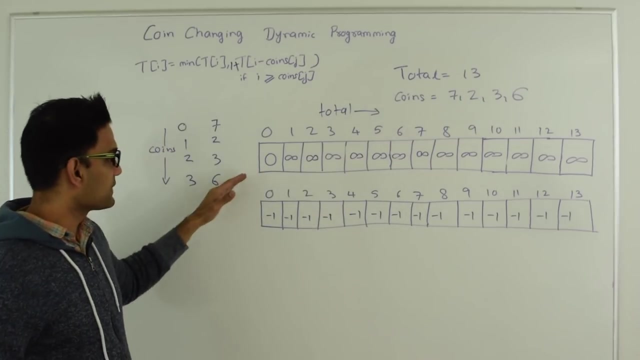 you are picking the jth coin. So the minimum of picking the jth coin or not picking the jth coin will be T. So next let's apply this formula on this example here. So here we are going to take two one dimensional array of lengths, total plus 1.. The first array is going to keep the minimum. 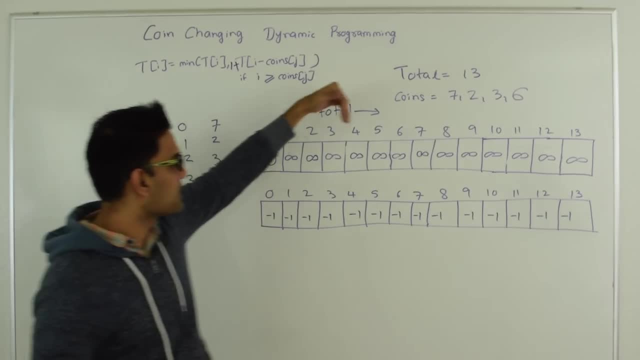 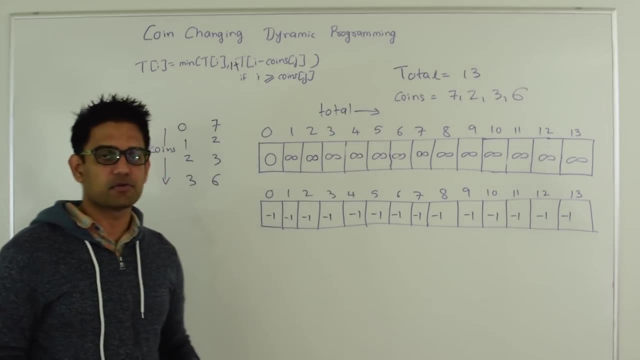 number of coins it takes to form the certain value. so T is going to store the minimum number of coins it takes to form total 5, while second array is going to be useful to get the final answer. Also, we are going to iterate through these coins one by one and apply this formula Here. 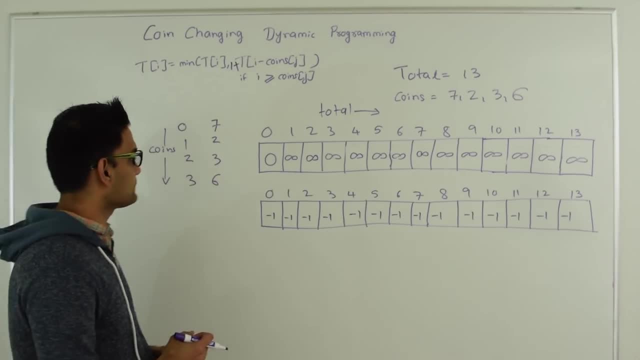 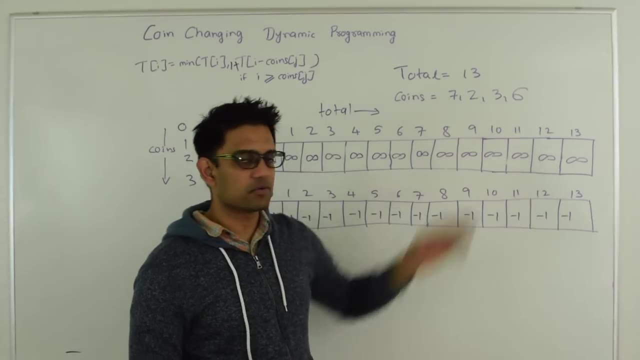 you can see that the coins are not in a sorted order. Also, the value of T is 0 because it takes 0 coins to form total 0, while from 1 to 13 the values are infinity because we don't know how many coins it takes to form those total. 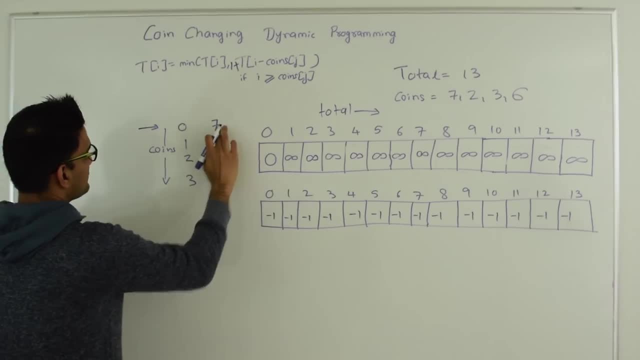 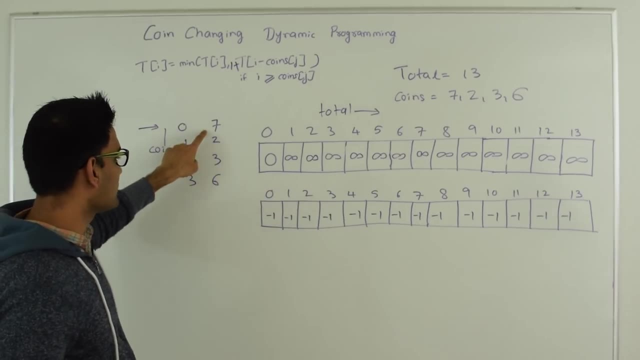 So first we start from 0th coin, which is 7. So j is 0 and i is going to be 1. So this is 0. So here total 1 is less than 7.. So no matter what we do, you cannot form 1 with just. 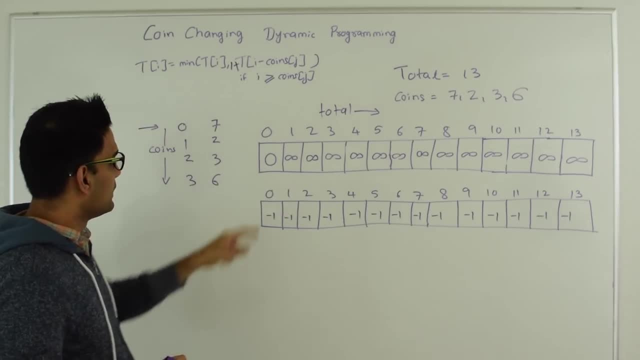 with one coin 7.. So we leave this as infinity. Similarly 2,3,4,5 and 6.. No matter what we do, we cannot form those total with just coin 7. So we leave them as is and move on to 7.. 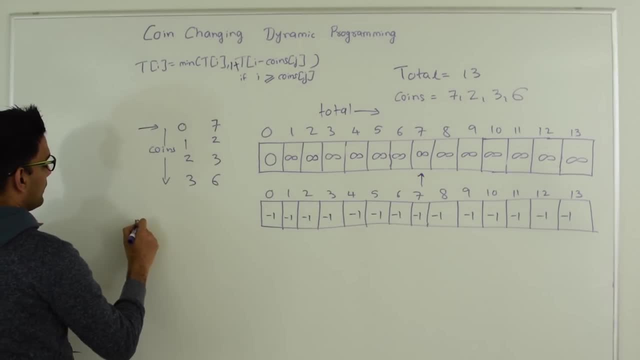 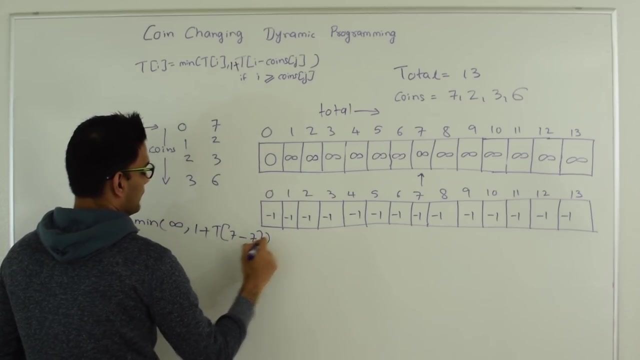 So here, applying this formula- minimum of whatever is in here, so infinity- or we are going to get or 1 plus T of 7, minus this denomination 7.. So this is infinity, or 1.. So this value 1 is less, So this value becomes 1, and in here I'm going to say that we reached this 7 from. 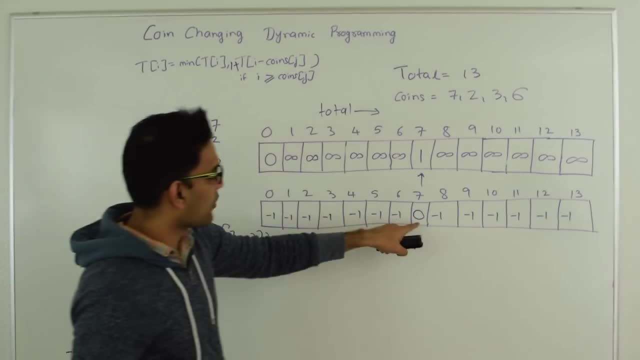 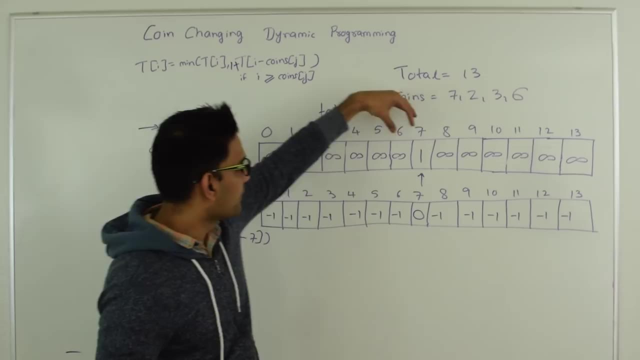 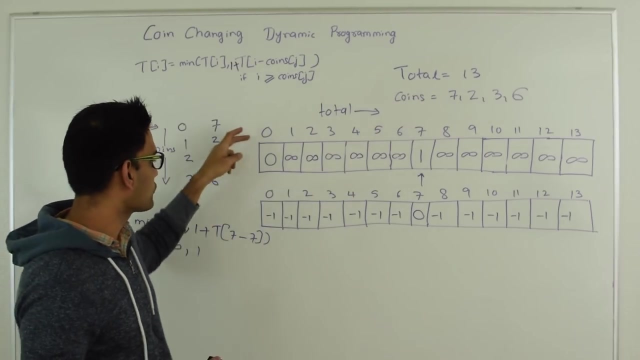 the coin of denomination,0th coin, which is of denomination 7.. So this value is 0, indicating that we picked 0th coin. So again here, as you can see, when we picked the coin of denomination 7, then we are left with 7 minus 7.. So 0th total, and we know that it takes 0 value to form 0 total, which is: 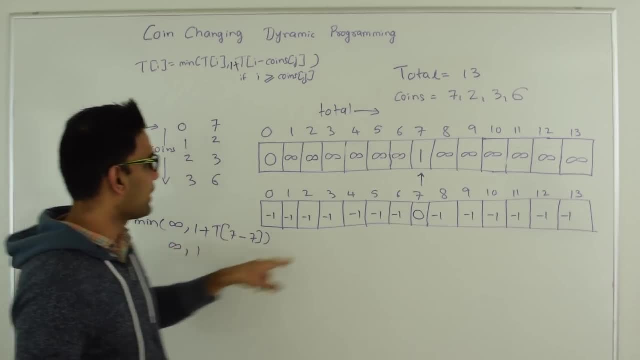 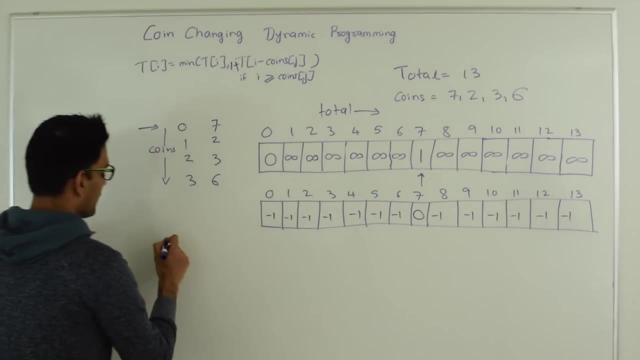 why T, of which is why 1 plus 0, that value is 1, which is why this value, 1, is here. Then we are going to move on to 8.. So to get 8, we have minimum of infinity, or T of 8 minus. 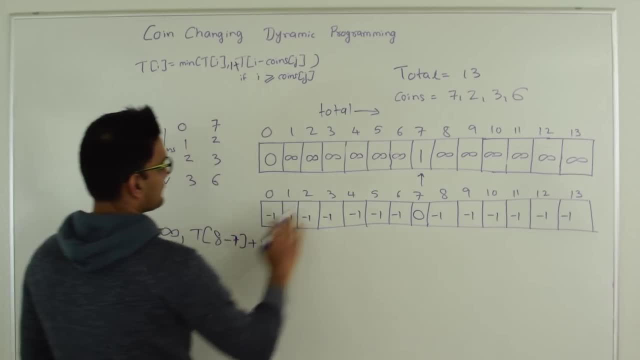 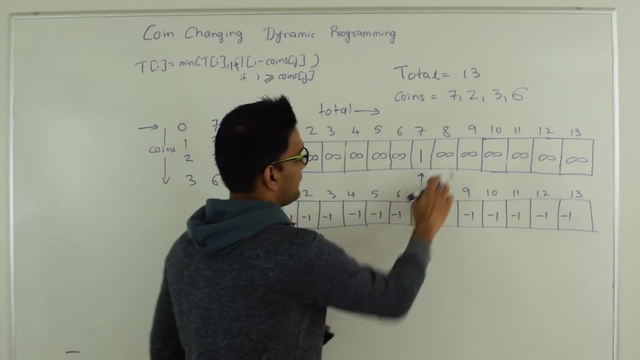 7. So 8 plus 1.. So this is T of 1.. This value is infinity, So infinity plus 1 is infinity. So 8 doesn't change and it stays infinity. Similarly 9,10,11,12 and 13.. All those values. 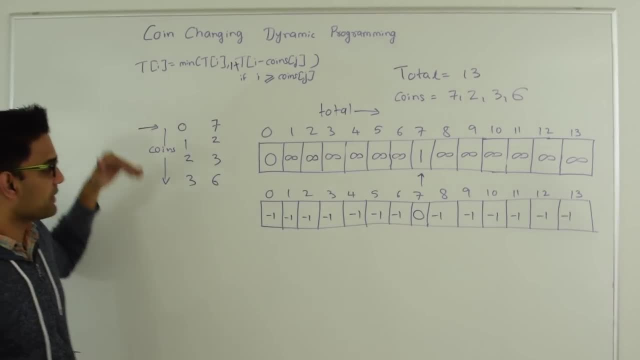 will not change. So, as you can see, after I'm done with the 7, there is only total 7 which can I form with 1 coin, while rest of the total I cannot form. So then we are going to pick the next value. 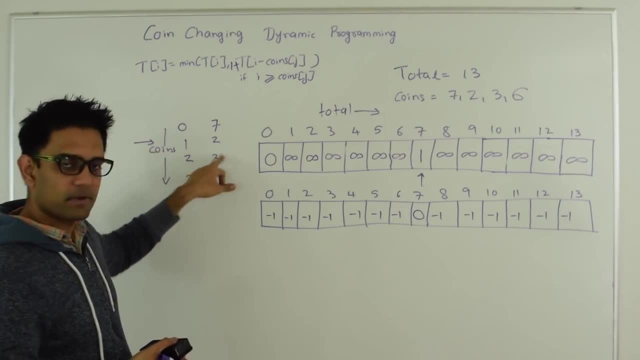 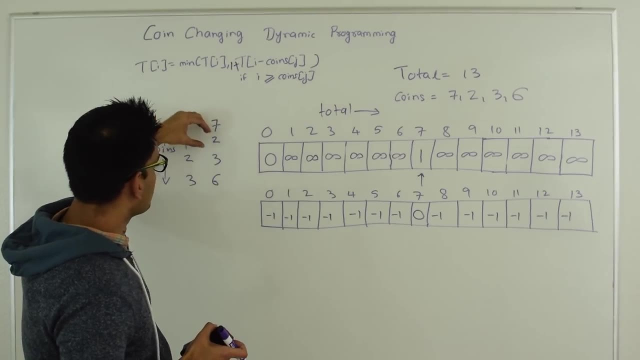 Which is index j 1 and the denomination of that coin is 2.. So again, starting from here, the total is 1 and the denomination of the coin is 2, and we cannot form 1 with coin 2 or 7. so this: 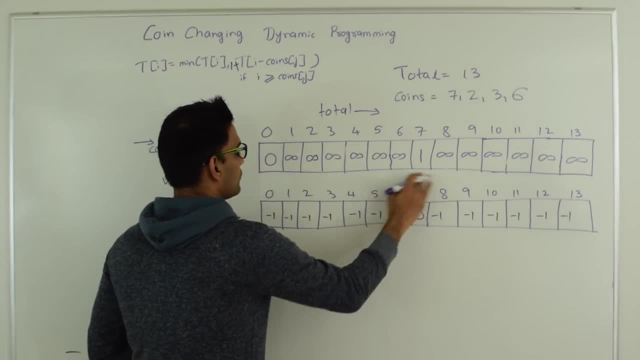 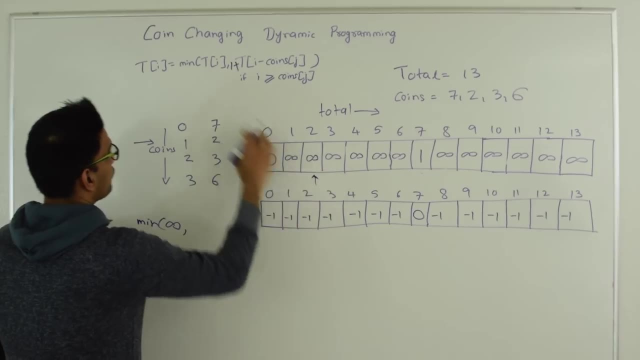 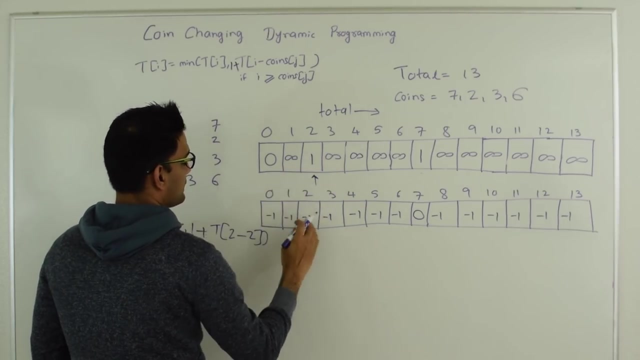 stays to be infinitycontinues to be infinity and we come to this point. So again to form this guy, minimum of either infinity or whatever is stored here. so minimum of T of i, or 1 plus T of minus this coin, 2, so this value is 1 plus 0, so this is 1, and here I'm going to 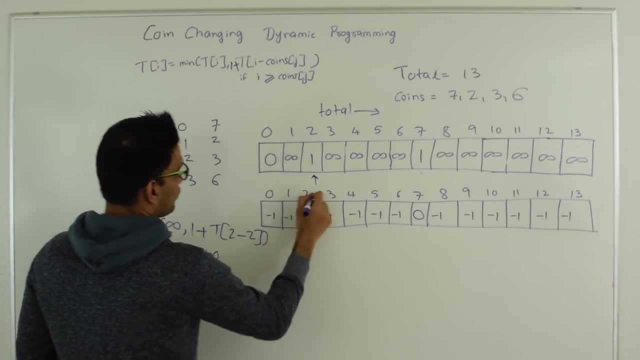 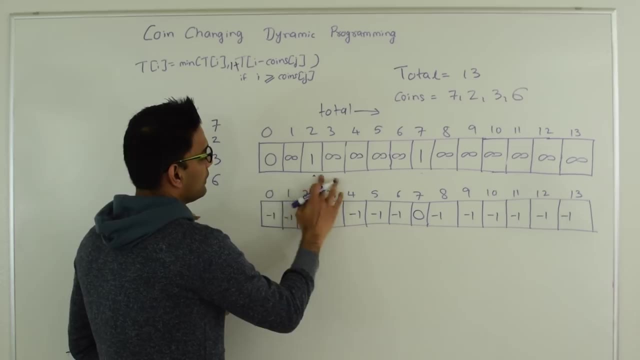 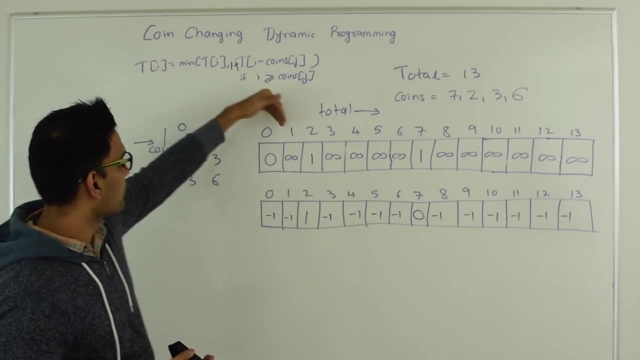 indicate that I used coin 1 to come to this value 2.. Then we are going to go to 3.. For 3 also we cannot. since we cannot form 1, we cannot also form 3, because 3 minus 2 is. 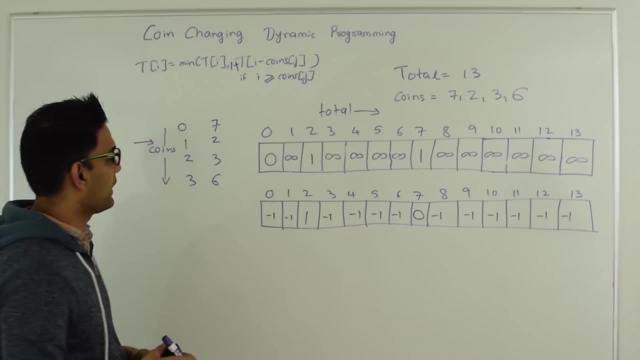 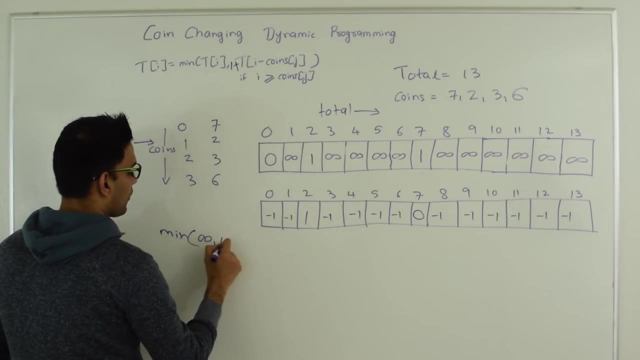 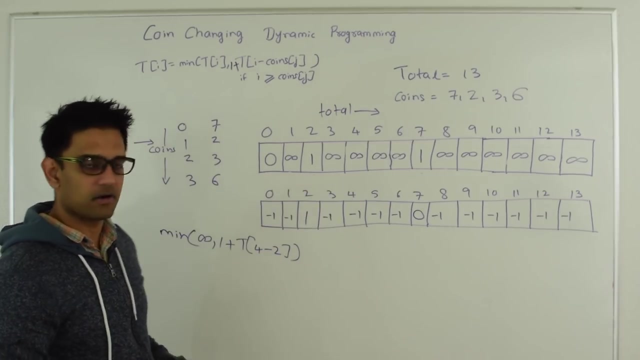 going to be 1 and t of 1 is infinity. so we cannot do anything better than infinity For 4, minimum of infinity, or 1 plus t of 4 minus 2, so to form form total 4 with coin 2, if we subtract 4 from 2 we'll horrific and we 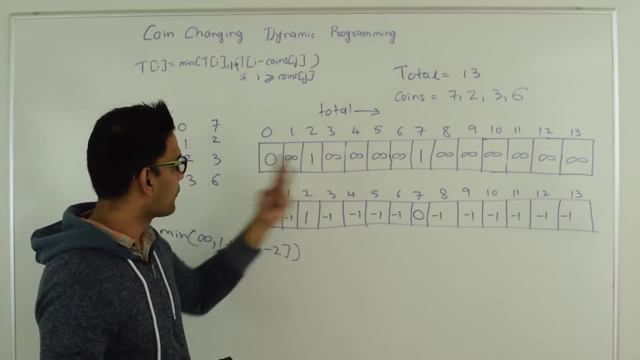 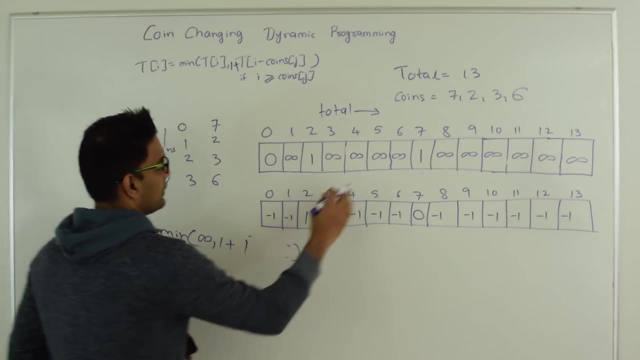 already know that we can form 2 with one coin. so we can form 4 with 2 coins, which is 1 plus 2, which is 1.So 1 plus 1, which is 2.So this value here becomes 2.And here also I am going. 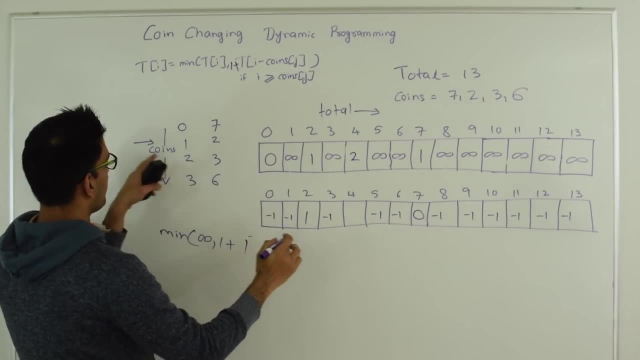 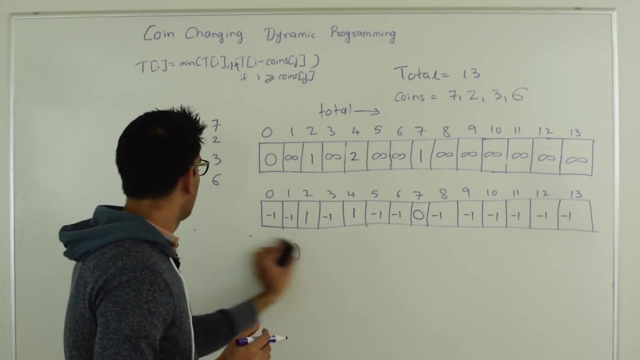 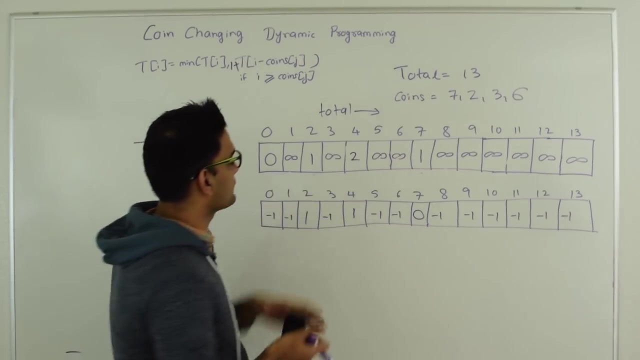 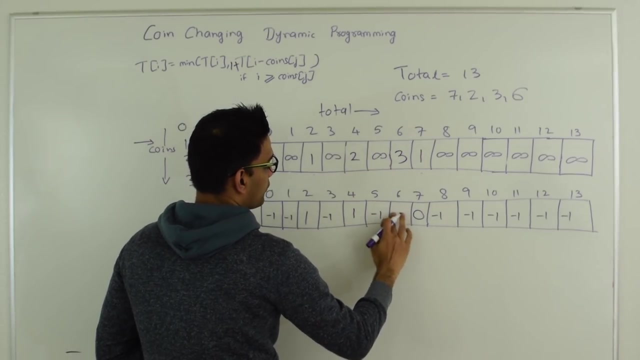 to indicate that I reached 4 from coin by picking coin 1, which has denomination value 2.Then we are going to go to 5.Again, 5 cannot be formed because 3 cannot be formedSo we go to 6.So 6 can be formed by 2 plus 1 coinSo this is 3.And here also, I am going 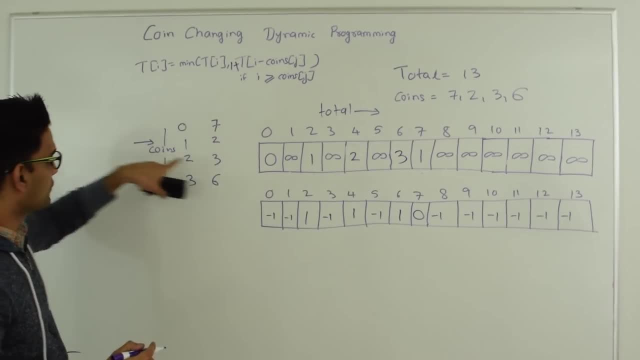 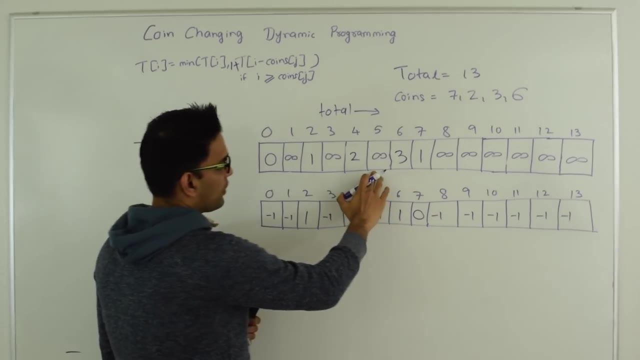 to put a value of 1 because we picked this 1th first cointhis 1 coin which has denomination 2.Then 7 isagain, 5 cannot beagain, 5 is not formed and 7 already has this minimum 1 coinSo 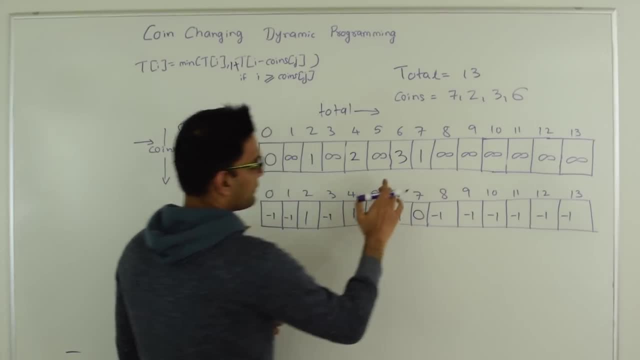 we cannot do anything betterSo we go to 8.To form 8, we go to 3 plus 1.So 4 plus 1 is 2.And here we are going to indicate that we picked coin 1.Then to get 9. we have minimum. 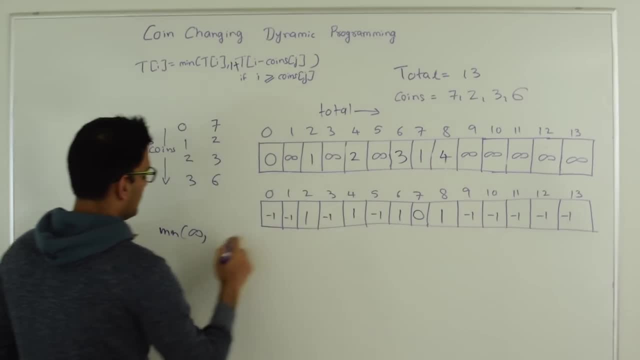 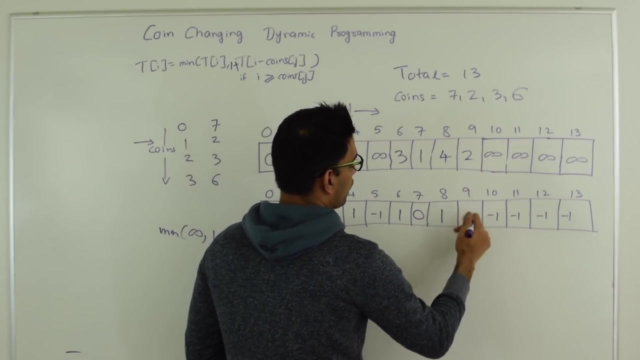 of infinity and 1 plus t of 9 minus 2.So t of 9 minus 2 is t of 7.So this value, 1 plus 1, is 2.So we can form 9 with 2 coins, and here I am going to say that I picked coin 1.So. 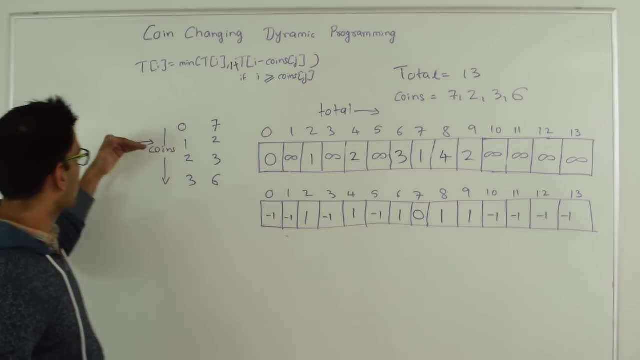 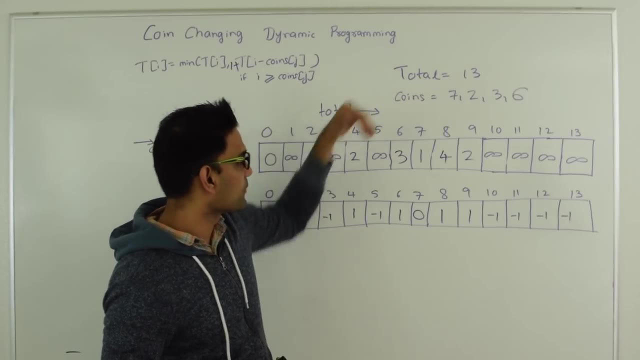 again to form 9.. We know that we are on the current coin whose denomination is 2.So if we subtract the value of 2 from 9, we are left with 7, and we know that we can already form 7 with 1 coin of. 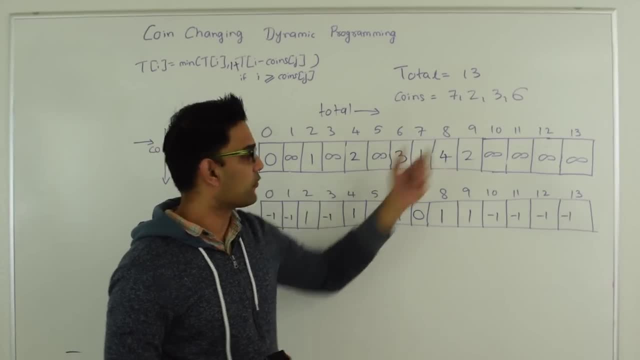 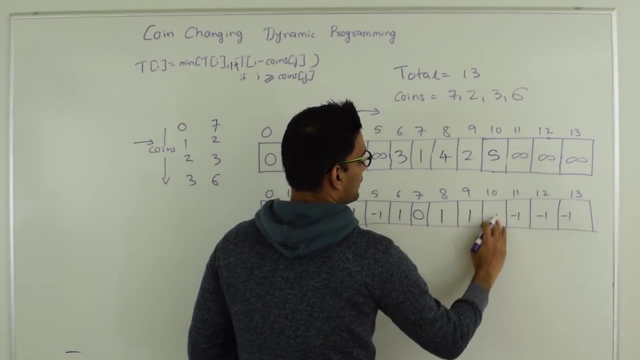 7.So that's how we end up having 2 coins to form total. 9.10 can be formed with 4 plus 1,5, and this value here will also be 1, indicating that we picked coin 1 to form 10.11 can be. 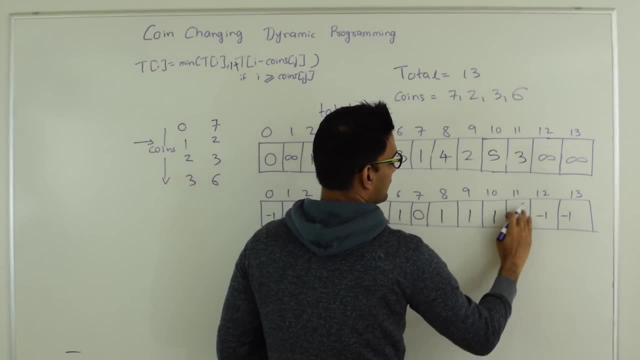 formed by 2 plus 1,3.. And here we say it is 1.12 can be formed by 5 plus 1,6, and this value is 1.And 13 can be formed by 3 plus 1,4, and this value is also 1.So after we are done doing 2, we can. 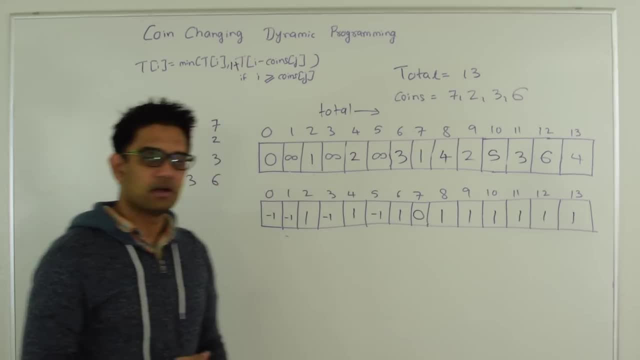 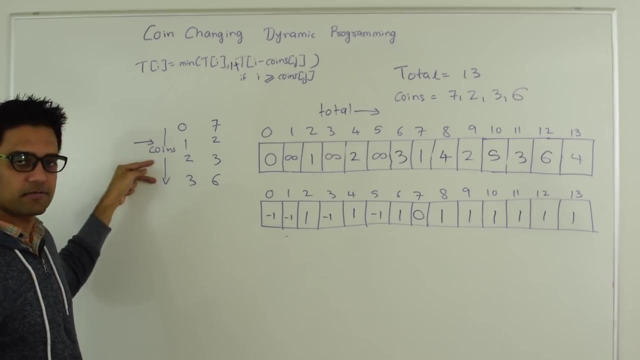 form 13. but it takes 4 coins to form total value 13 if we just pick among coins with denomination 7 and 2.So next, let's do remaining of the 2 coinsSo let's do remaining of the 2 coinsOur next coin has denomination 3.So if the j is 2 and denomination is 3.So again, 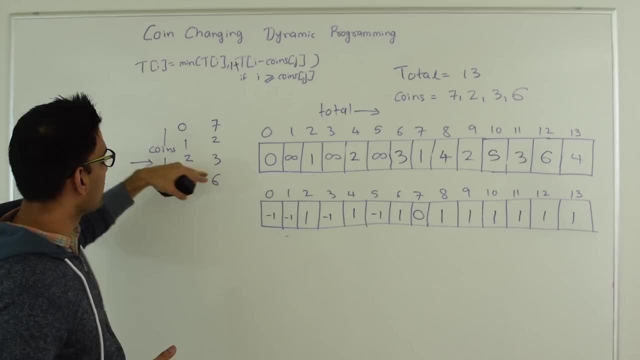 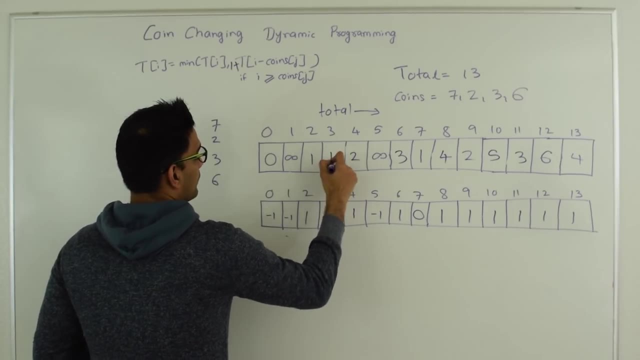 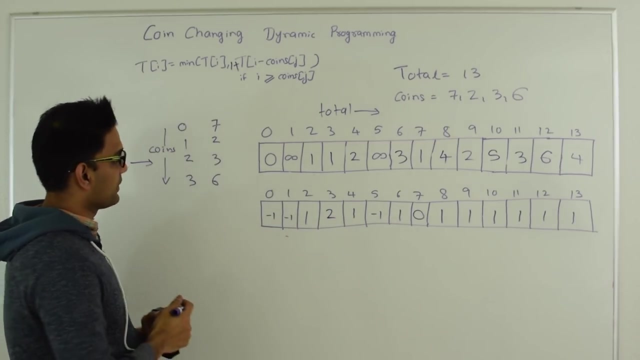 starting from 1,1 cannot change, because total is 1, which is less than 3, so we cannot do anything about it.2 cannot changeFor 3, this value becomes 1.And here we will indicate that we got 3 by picking second coin whose denomination is 3.Then 4 to form 3.So we can. 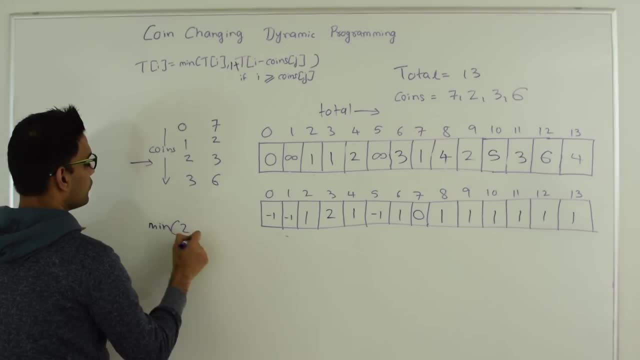 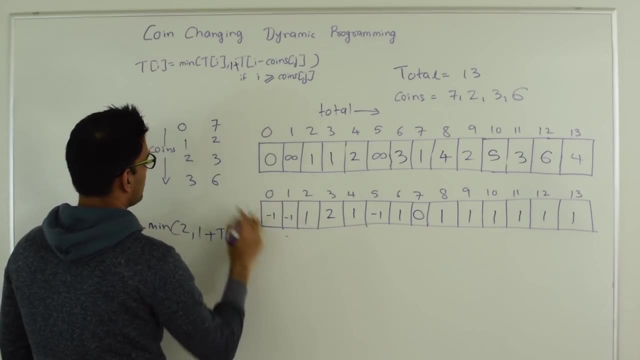 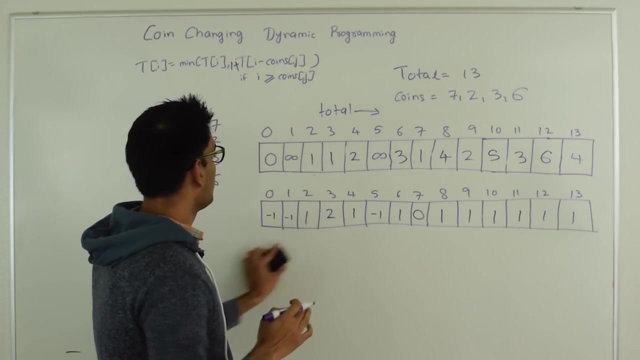 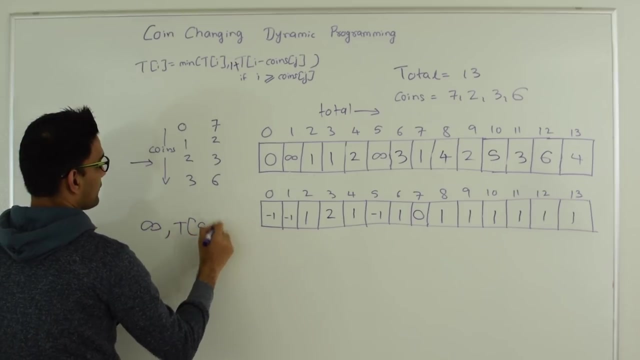 to get 4, either minimum of 2 or 1 plus t of 4, minus this 3.. So this is t of 1. t of 1 is infinity, so we cannot do better than 2.So we leave it as thisFor 5 we have minimum of infinity, or t of 5 minus this current coin, 3 plus 1.So. 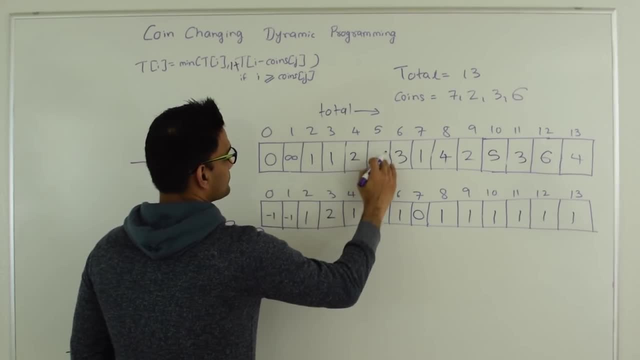 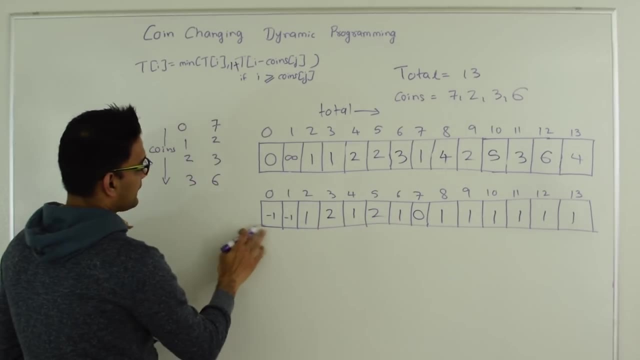 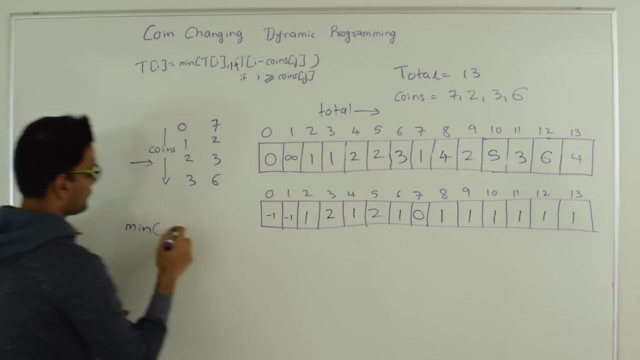 t of 2 is 1.. so this value will become 2, and here I'm going to indicate that I picked coin 2.. For 6, for 6 we have minimum of current to form 6, which is 3 coins or 1 plus T of. 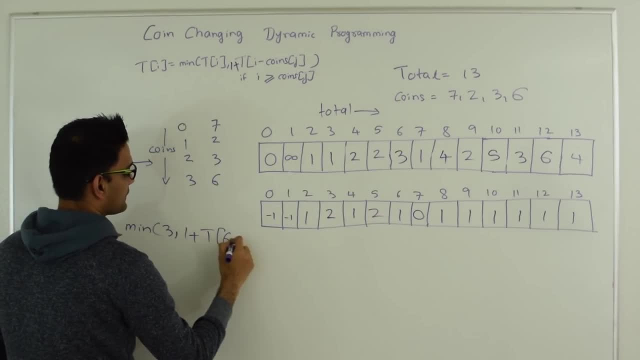 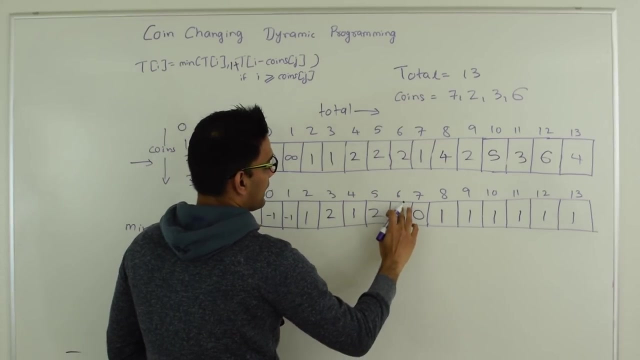 6 minus this denomination. so 6 minus 3 and 6 minus 3 is T of 3 and T of 3 is 1. so minimum of 3 and 1,1. so this is this value is 2.. So we change this to 2 and in 6 we. 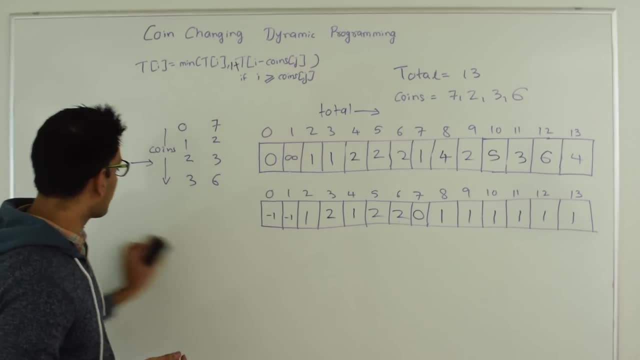 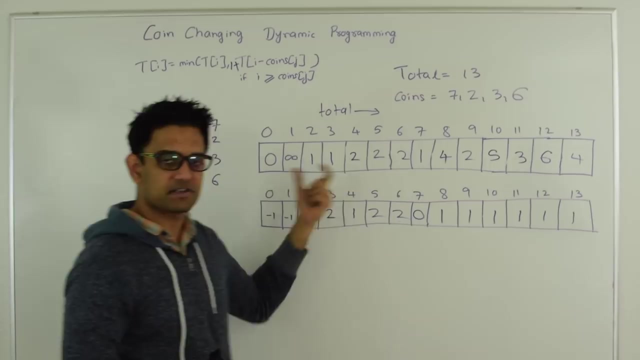 said, we pick coin 2.. So before, before 3 was introduced, it took total of 3 coins to form 6, which is 3, 3 coins of value 3. but now that this third coin, which has a- now we have a coin whose denomination 3- got introduced, we can form 6 in just 2 coins. 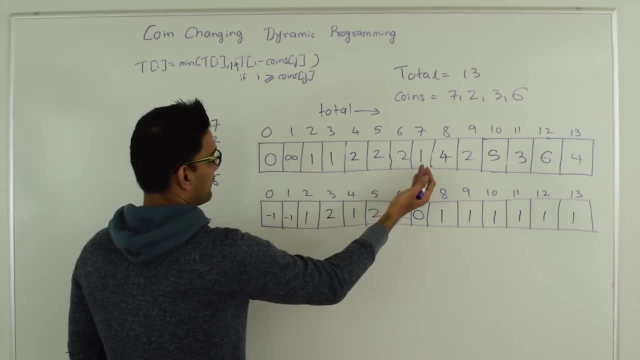 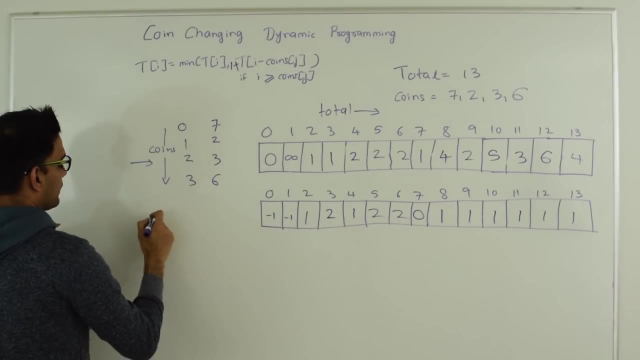 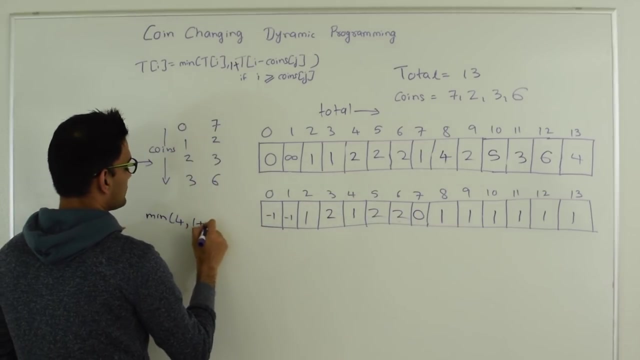 which is why this got updated. Going to 7, I mean we cannot do anything better than 1, so let's go to 8.. So for going 8, we have minimum of 4 and 1 plus T of 8 minus 3. so T of 8 minus 3 is 5. 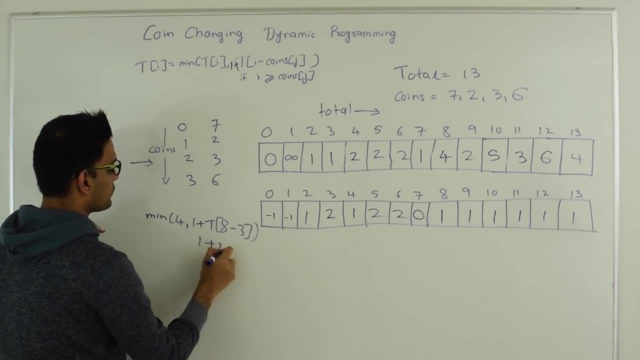 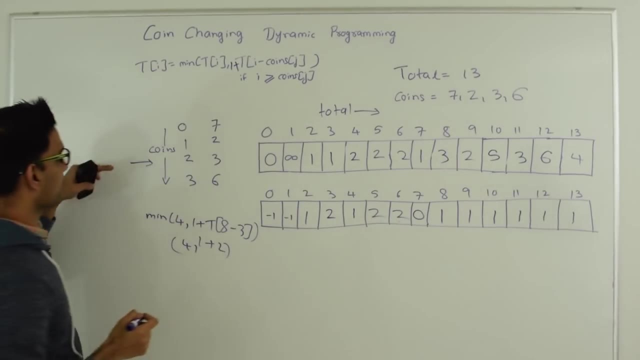 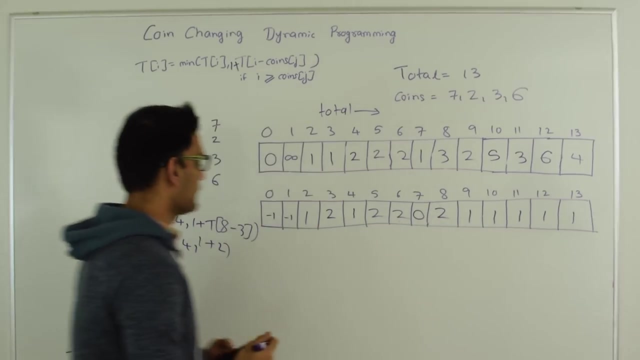 which the value here is 2, so 1 plus 2, or 4, so minimum is 3, so 8 becomes 3.. So before, before this coin of denomination 3 was introduced, it take 4 coins. but now we can do it in 3 coins and we'll indicate that we pick this second. second: 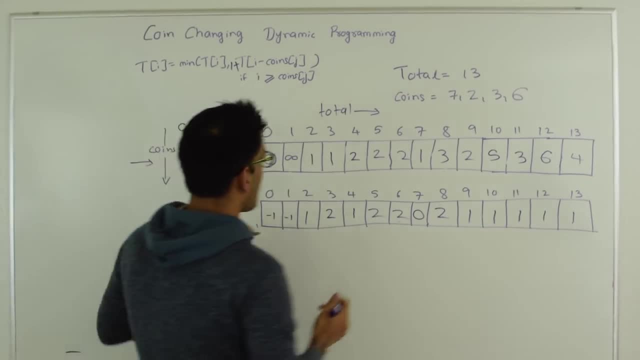 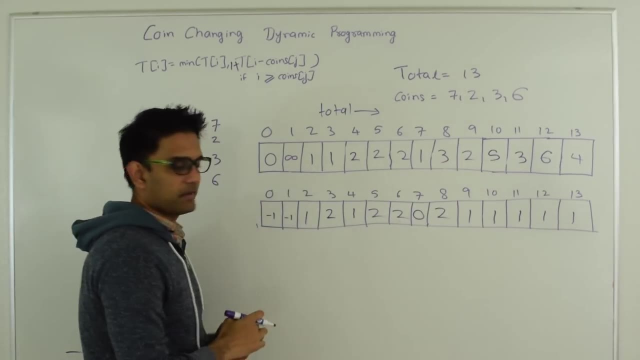 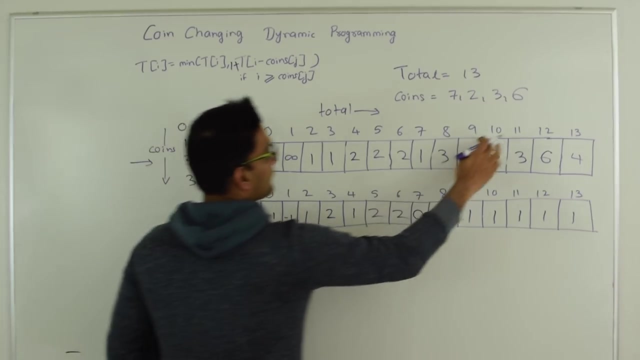 index coin Going to 9,. 9 will be a T of 6, so 2 plus 1, 3. that's not going to be better than 2, so we leave 9 as is For 10 minimum of 5 or 1 plus T of 10 minus 10. 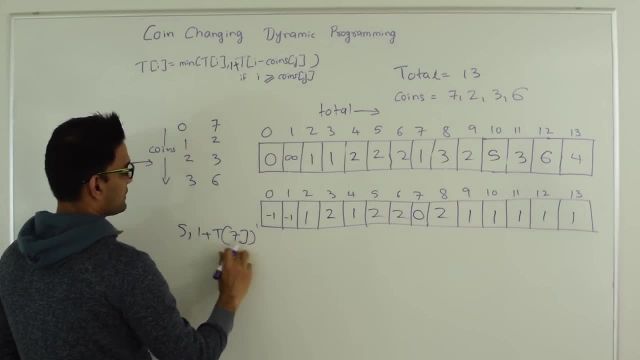 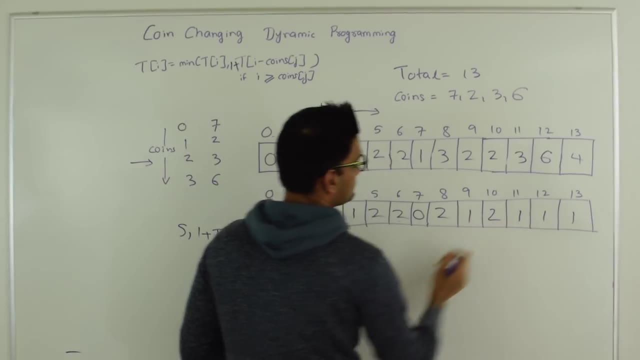 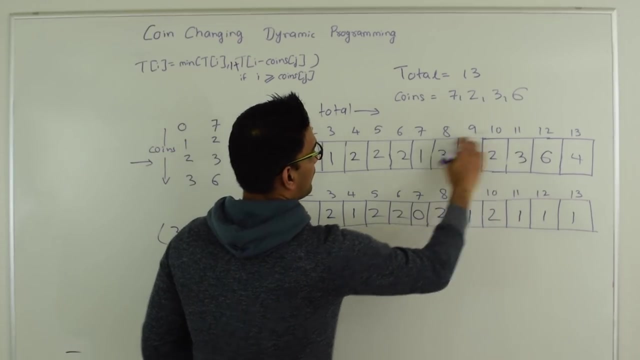 minus 3, which is 7.. So T of 7 is 1, so this value becomes 2 and we're going to indicate that we picked second coin. For 11, we have value 3, minimum of 3 or 11 minus so 11. 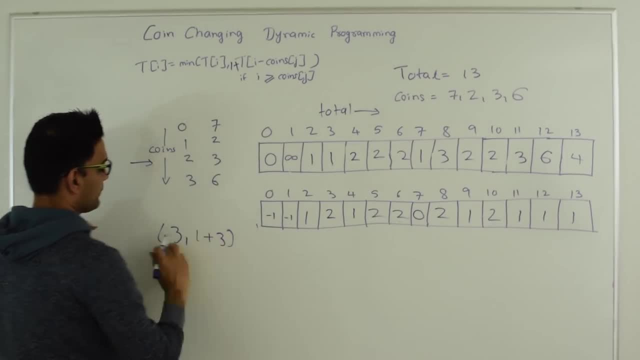 minus 8, which is 3, so 1 plus 3. so minimum of this is 3, so 11 doesn't change this 12. we have minimum of 6 or 1 plus T of 12 minus 3, 9, so T of 9.. T of 9 is 2, so 1 plus 2 is 3, so 12 can now be. 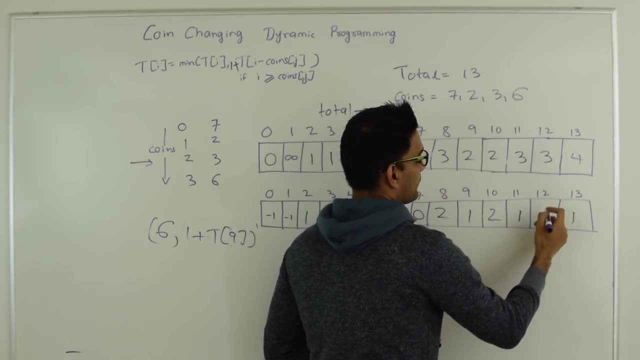 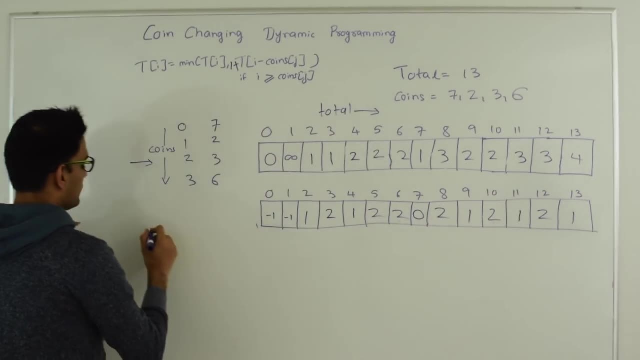 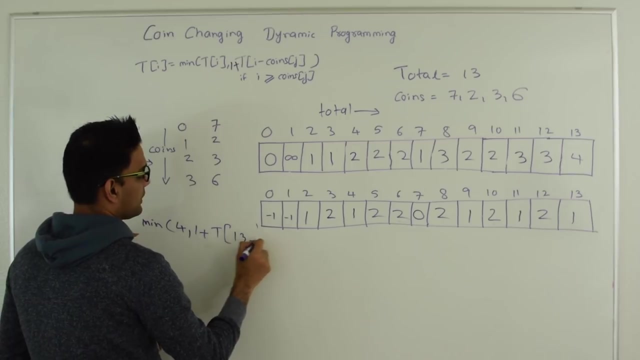 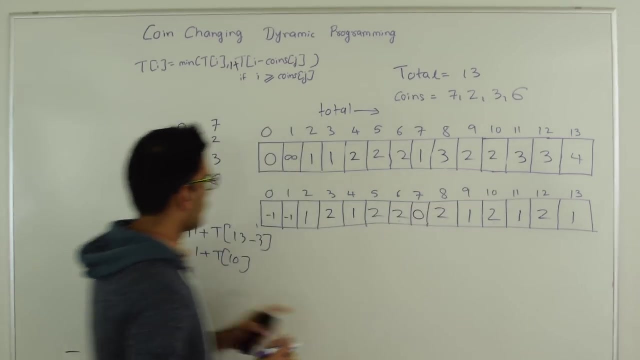 formed in 3 coins, and here I'm going to say that I picked coin of index jth 2.. And finally, 13,. minimum of current value of 13,: 4 or 1 plus 30 minus 3, so 1 plus T of 10, so T of 10 is 2, so 1 plus 2 is 3, which is: 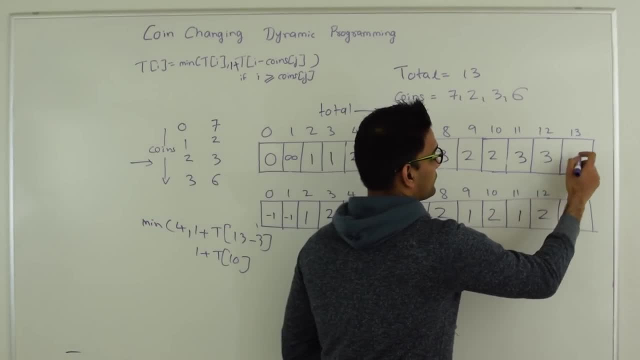 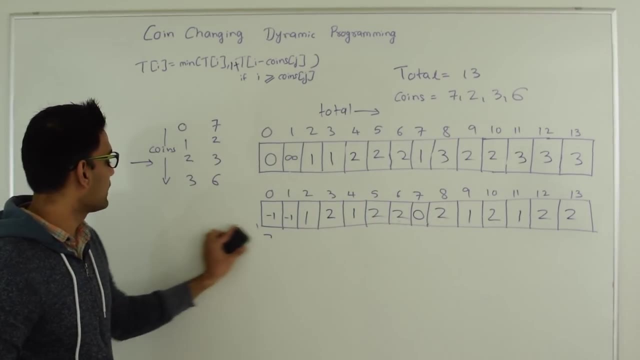 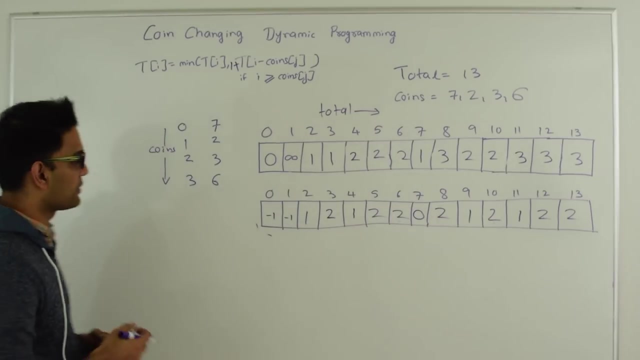 greater than, which is less than 4, so this value becomes 3, and I'm going to say that I picked J2.. So, after this second coin is done, this is what we are left with, and this is the minimum number of coins it takes to form 30. So, finally, 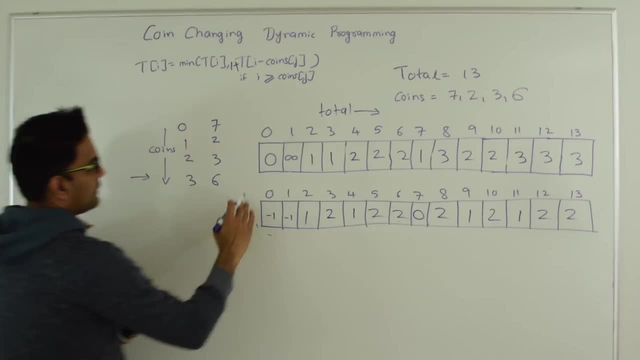 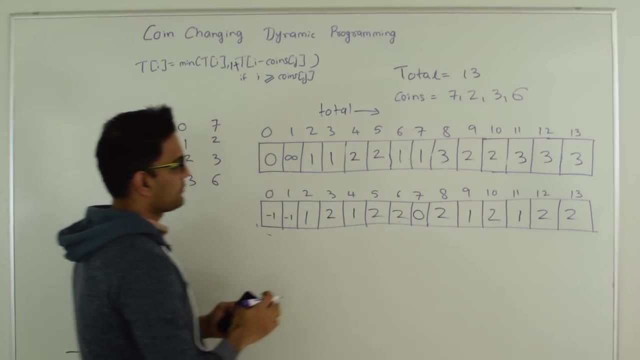 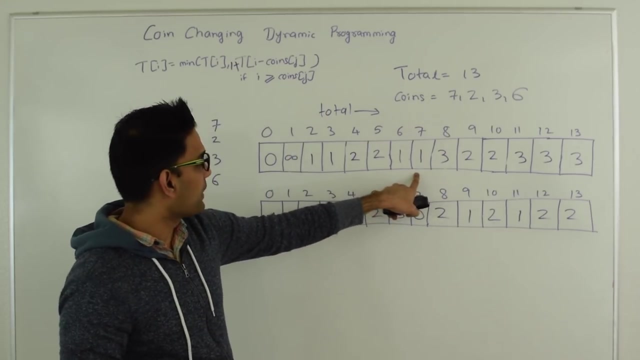 let's pick this coin with denomination 6.. So till 5, we cannot do anything. This guy here will now become 1, because it can take just one coin of 6 to form this, and we are going to indicate that we picked J3.. Then 7. we cannot do better than 1.. This 8 will now. 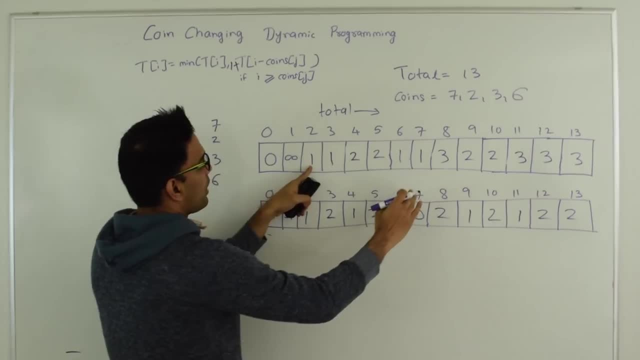 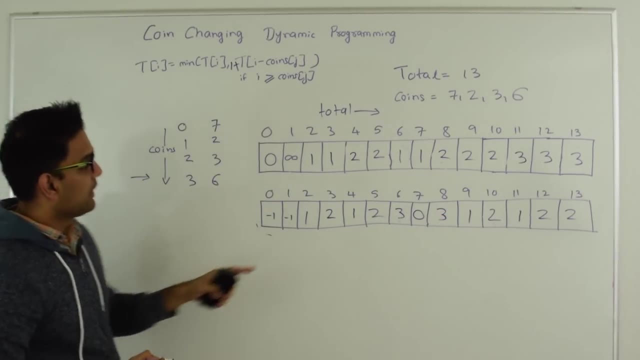 become 8 minus 2, which is 1. so 1 plus 1 is 2, and we are going to indicate that we picked coin 3.. And for 9, you cannot do better than 2. yeah, you cannot do better than 2.. 10, you cannot do. 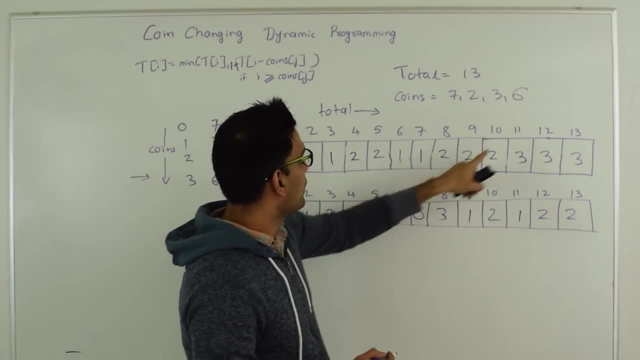 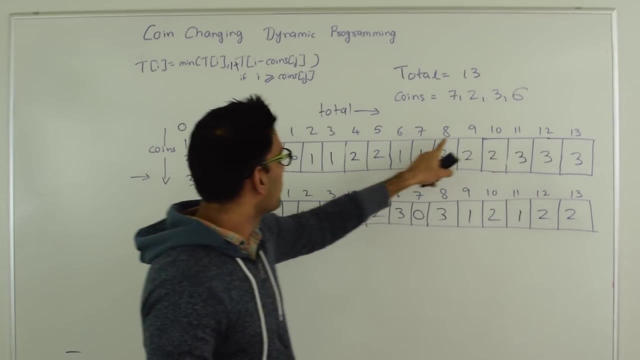 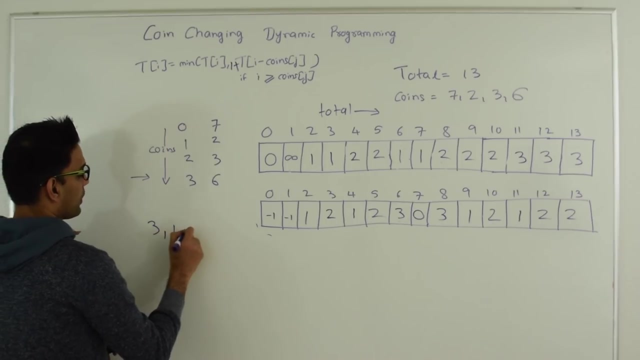 better than 2.. 11, you cannot do. 11 minus 6 is 5, so 2 plus 1 is 3, so you cannot do better than 3.. 12.. 12 minus 6 is 1, so either minimum of 3 or 1 plus T of 12 minus this 6. 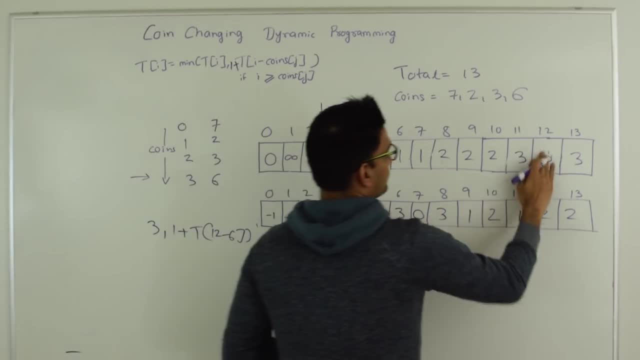 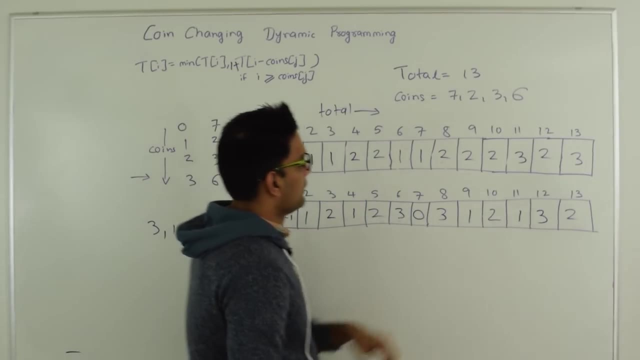 and this value is 6, so that value is 1.. So, yes, we can do 12 in 2 coins, and this here we picked 3.. And finally, 13.. 13 is 30 minus 30 minus 30 minus 6 is: 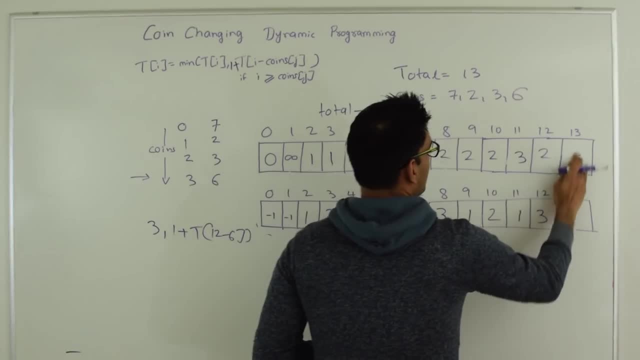 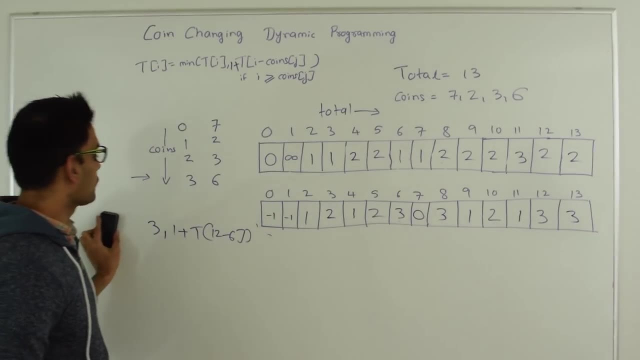 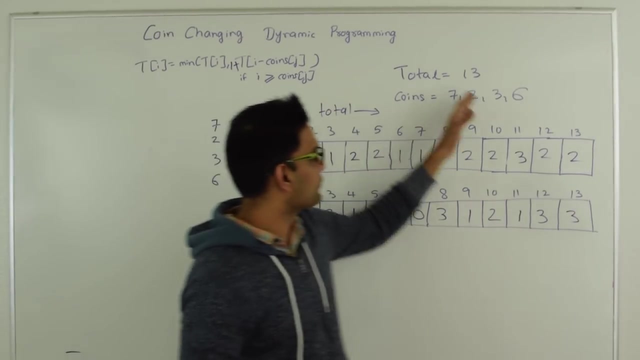 30 minus 6 is 7, so we can do 13 also in 2 coins. and here we are going to say that we picked total 3.. So this is the minimum number of coins. 2 is the minimum number of coins it takes to form total 13.. So next let's see how we. 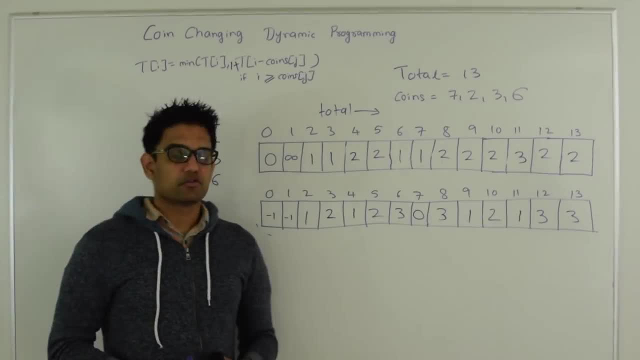 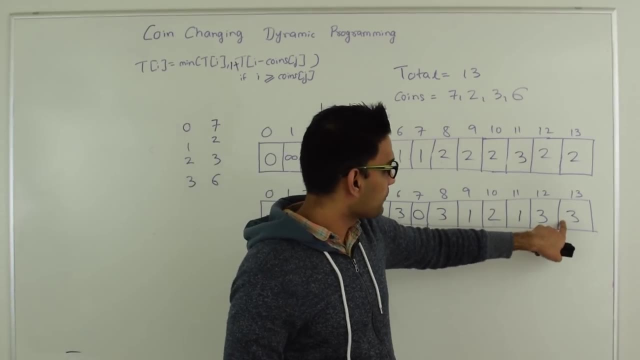 can find out what are the coins it takes to form total 30. So we know that we can form 13 with two coins. Let's see which are those coins. So we go here and we know that we picked third coin to form 13.. So we know that third coin is 6.. So we 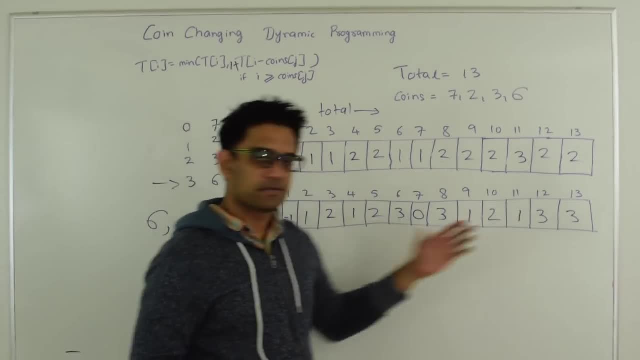 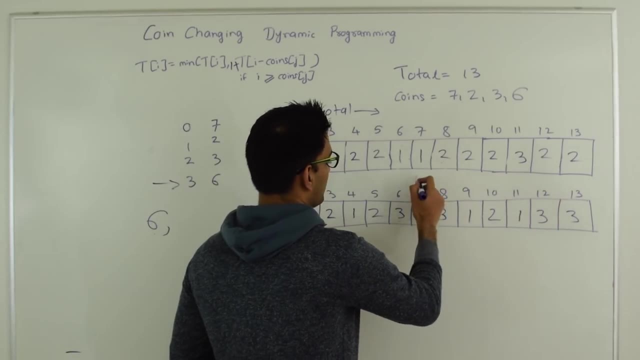 know 6 is in the answer. Then, since we are picking one coin of 6, we are left with 13 minus 6.. So 13 minus 6, we jump directly to 7.. And now we know that to get 7 it takes: 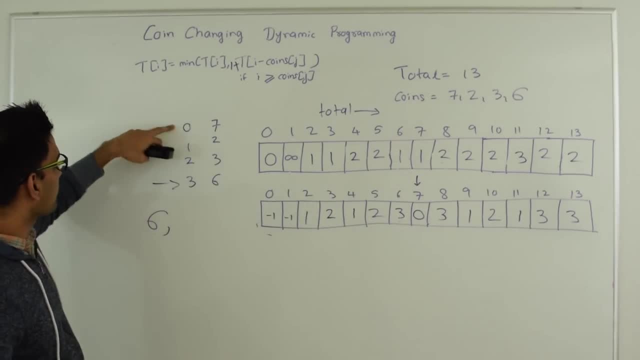 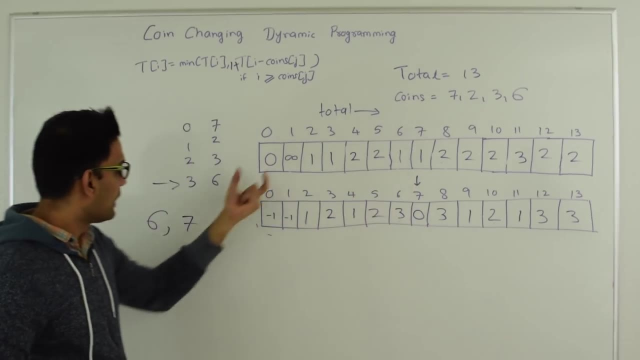 it took coin 0. So the value of coin 0 is 7.. So we come here and now, 7 minus this 7, we are left with 0, and then we reach this value, 0. and as soon as you reach this value, 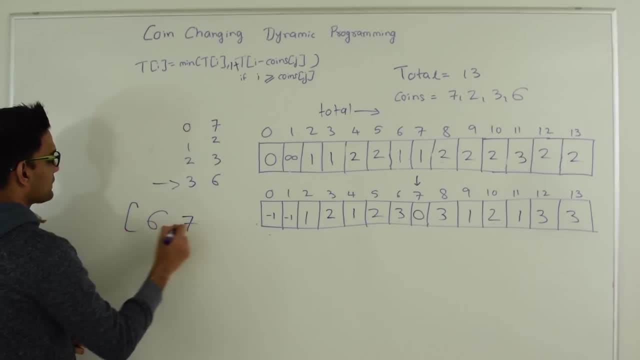 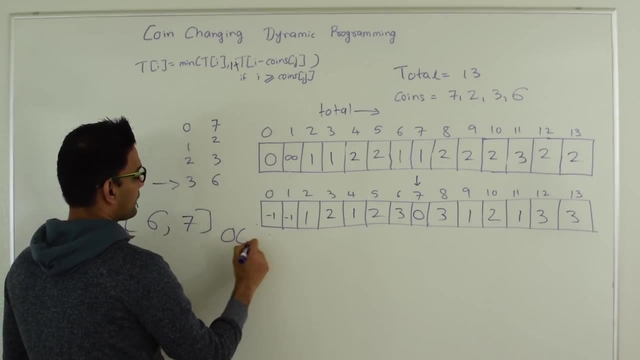 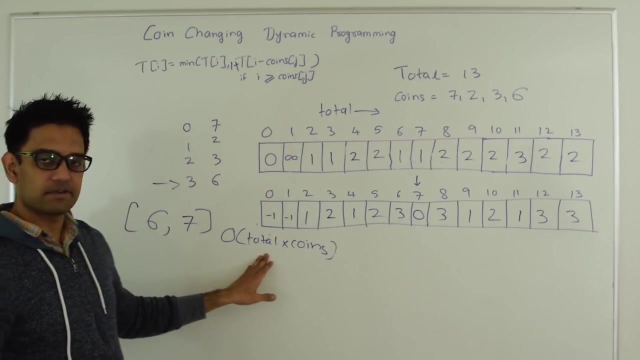 0. you know that you found your answer. So these are the two coins it takes to form total 30.. Let's do the time complexity. So the time complexity of this algorithm is total into number of coins. So, since total is not proportional in any way to the number of coins, this time 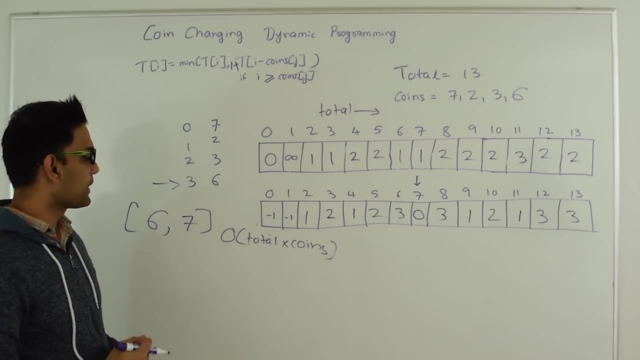 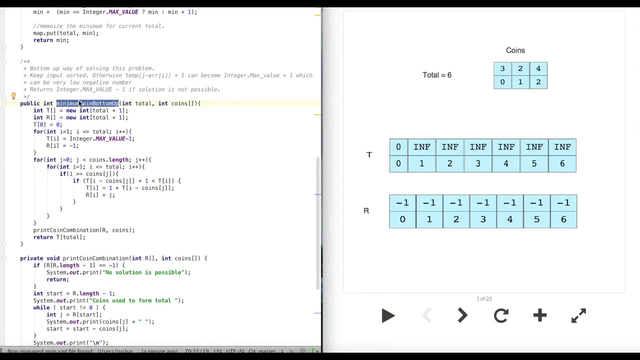 complexity is pseudo polynomial. Also, the space complexity is O. So next let's look at the code for this algorithm. The main function here is minimum coin bottom up In the example. our total will be 6 and the coins will have denomination 3.. 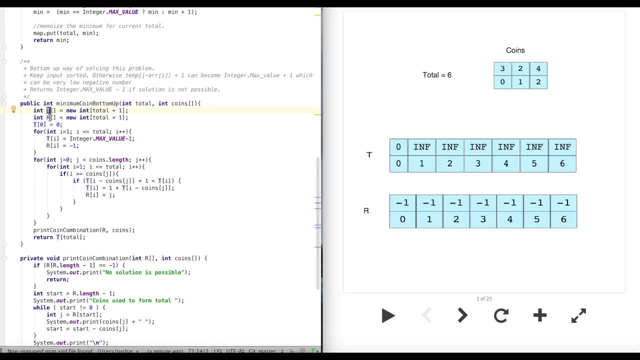 So the value of the value of the total will be 2 and 4. t and r are initialized as size of total plus 1. So in this case, going from 0 to 6 and 0 to 6. t of 0 is 0 because it. 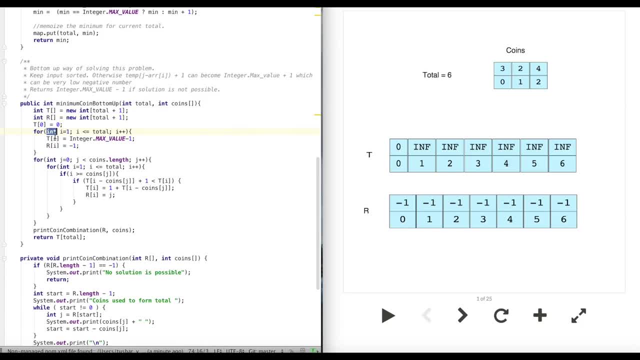 takes 0 coin to form total 0. And rest of the t, t of 1 till t of total, will have value infinity, as here integer dot, integer dot, max value minus 1.. And r of i is all minus 1.. Then 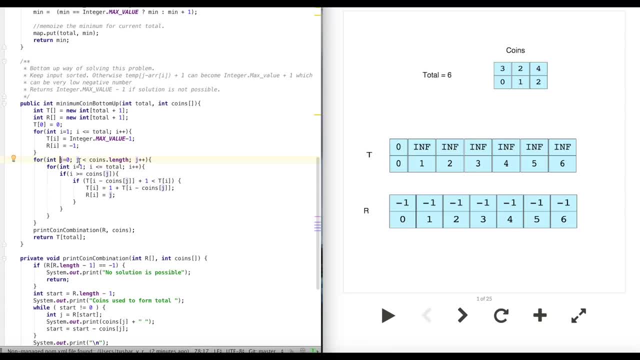 we'll take over our J will go from 0 to all the coins we have and for every J or I will go from 1 till the total value. so initially J is 0 and the denomination at coin 0 is denomination of a coin at 0 is 3 and I will go from: 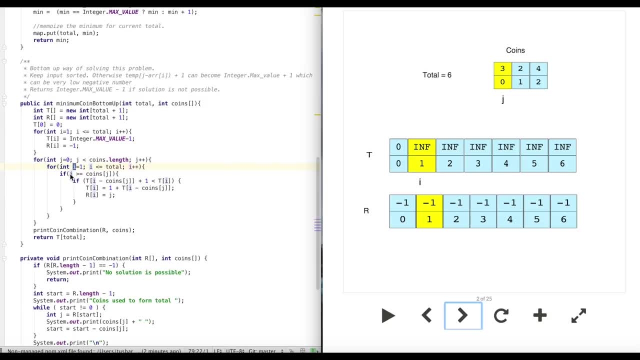 1 till 6. first we check is if I is greater than equal to coins J. if I is less than coins yet, then coin J cannot be used to form I. so there is no, no point doing anything. so only if I is greater than equal to coins J, then we do. 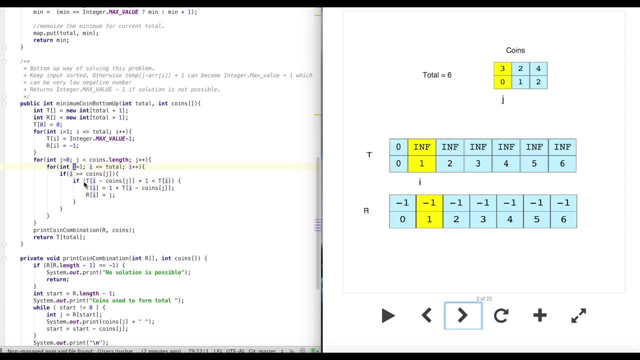 this: if I is greater than equal to coin J, then we have T of I is equal to T of I will be either be existing T of I or it will be. it will be minimum of either existing T of I or T of I minus coins of J. so in this case I is. 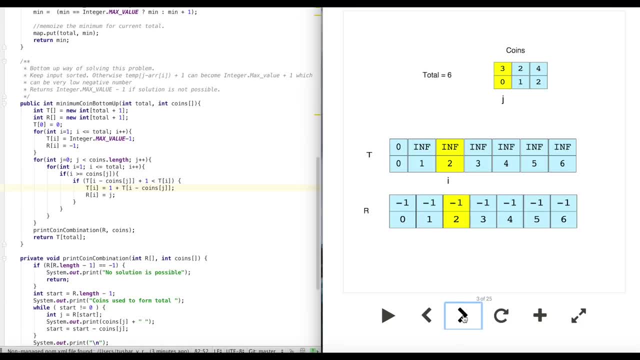 less than three, so we cannot do anything about it. then again, two is less than 3, so we cannot do anything about it. now, three is greater than equal to 3, it is so we go into this, if condition at T of I we're all, we're storing infinity, while T of I minus coins of J, which is 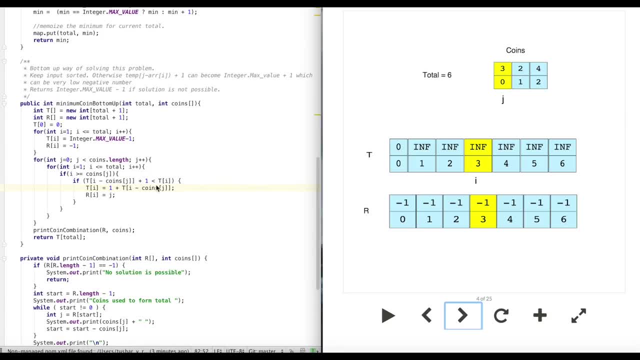 T of zero, we are storing a value 0, so this will be true. so we're going to store one, which is one, plus T of 0, which is 0. so at T of I, which is 3 of 3, we are storing 1, and r of i, which is r of 3, we are storing 0. 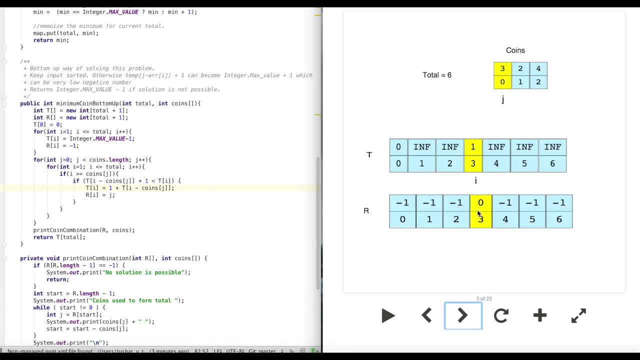 because j is 0, indicating that we used 0th coin to form total 3. then we move on to i equal to 4, and again we cannot. this cannot. we get a coin with denomination 3. doesn't help, because t of i minus coins of j, which is t of 1. this 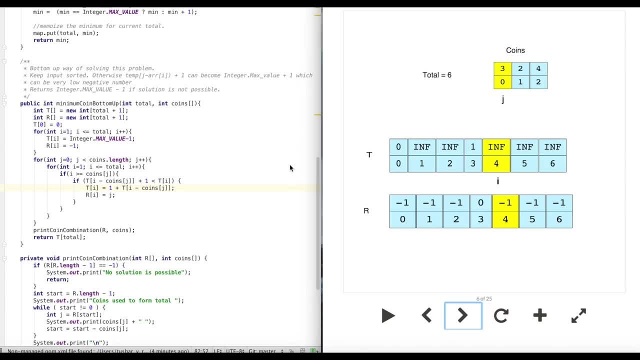 value here is infinity, so infinity plus 1 is not better than infinity. so there is no. this coin with denomination 3 cannot help. similarly 5 cannot help. and for 6 we can get 6 using two coins, because we can get 3 with one coin as we can get 6 with two coins. and at 6 also indicate that we 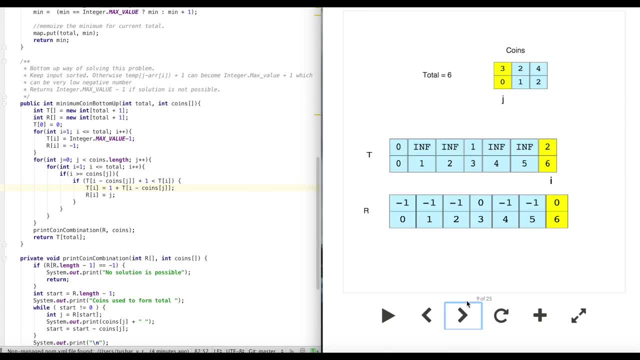 used 0th coin to form total 6. then our j will increment to the next value, which is 1, and i again will go from 1 to 6, as in this for loop. here again, 2 cannot here a 1 and i is 1 and coins of j is 2, so this cannot change anything. this. 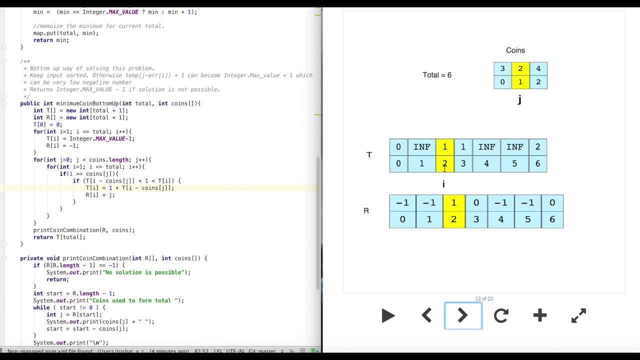 value now will become 1, because it takes one coin to form total 2, and we are also indicating that to form total 2 we are using a coin. 1 then 3. we cannot do better than already we have done, which is 1, so we don't change anything. 4: we. 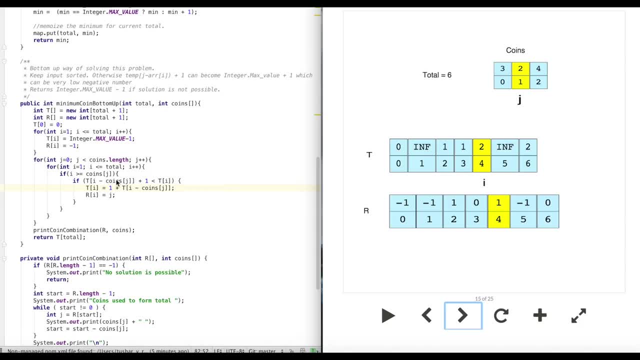 can now get into coins, as if you apply this exact, if this apply this formula here: five again we can get into coins, and six, we cannot do better than two. so at this point of time I as again reach the total. so again our for loop goes back to the. 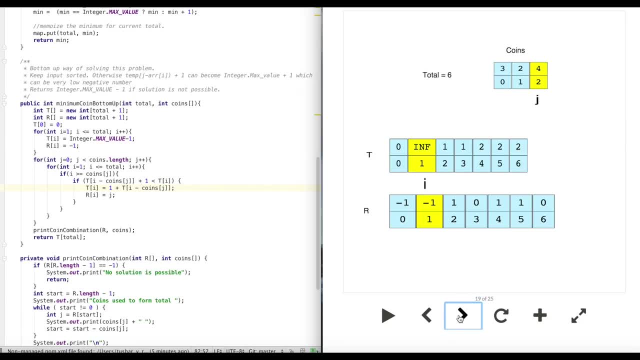 top and increment our J by one more, so J becomes two, and again I starts from one till total and again for cannot help but till three. at four now we can get total for with just one coin, so we'll indicate that we are using a point to get four. 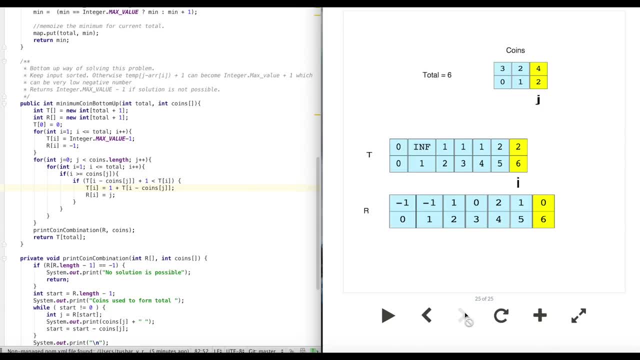 and this value here becomes one and five and six. we cannot do any better. so at this point of time the for loop terminates and we- this is our results. so to get six, it takes total of two coins and if you want to see which are those two coins, you can. 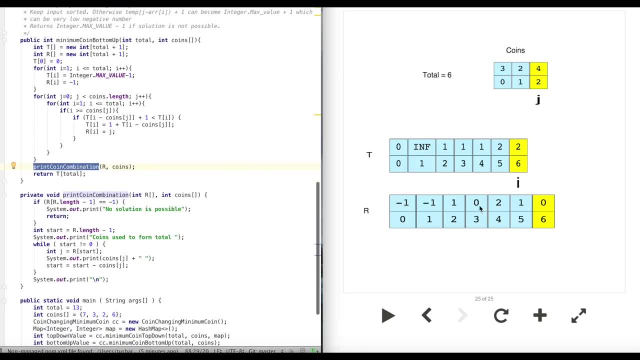 look at this function print coin combination. to get that you have to go into this our array and to see and see you, how do you form six? so six is formed with zero coin. so you need one coin of three and after you subtract three from six, you're left with three. so you jump to three in this our array and then you 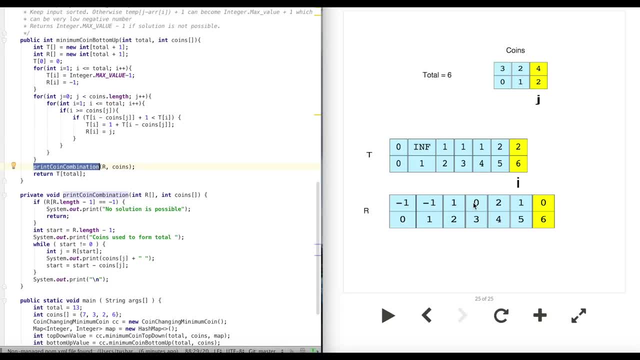 again need one coin of three, and then you subtract three from three and reach zero. so in total you took two coins of three to form total six, and all that logic is in this print coin combination. so this is all I have to talk about. a coin changing problem. the link to this. 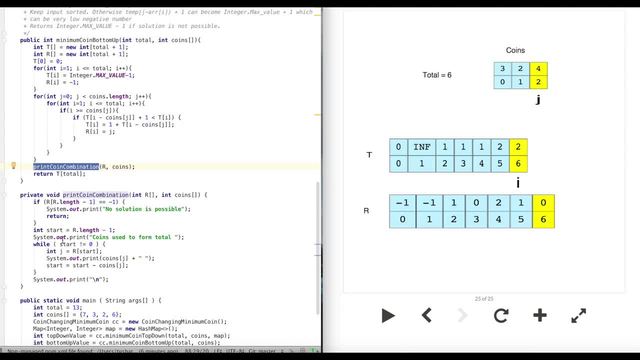 code, and python code is in the description section of the video. please like this video. share this video. comment on this video. check out my facebook page and check out my github link. thanks again for watching this video.